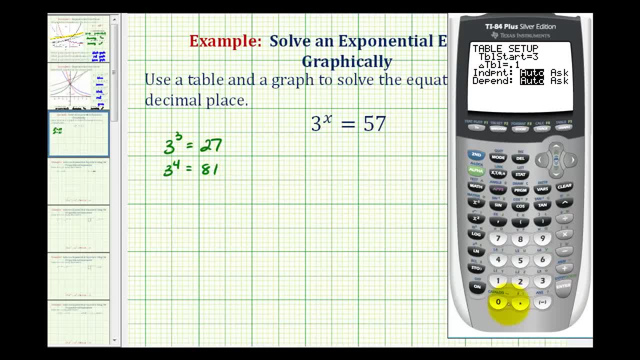 to one decimal point, we'll make the change in the table 0.1.. Now if we go to the table by pressing second graph, we're going to scroll down and find the x value that produces the y value that's closest to 57.. 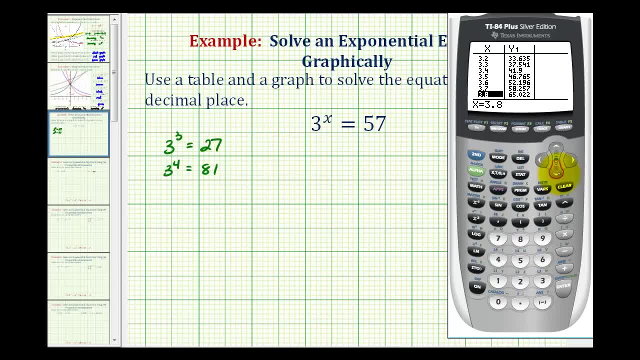 So let's go ahead and scroll down. Notice that x equals 3.7,. we have a y value that's approximately 58.25.. Now if we go to the table by pressing second graph, we're going to find that x equals 3.57,. 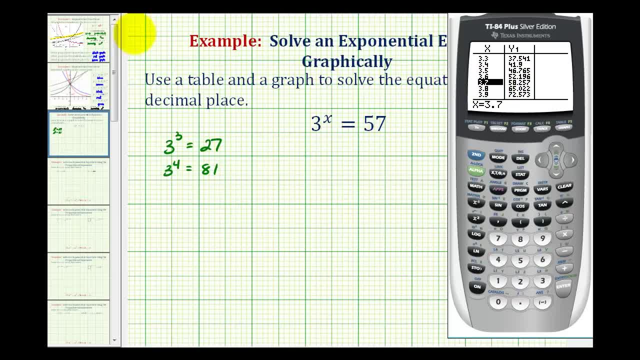 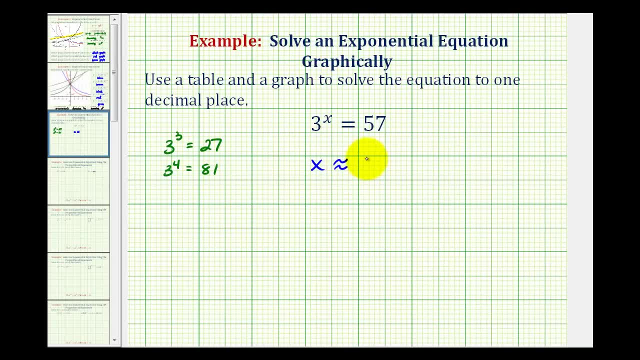 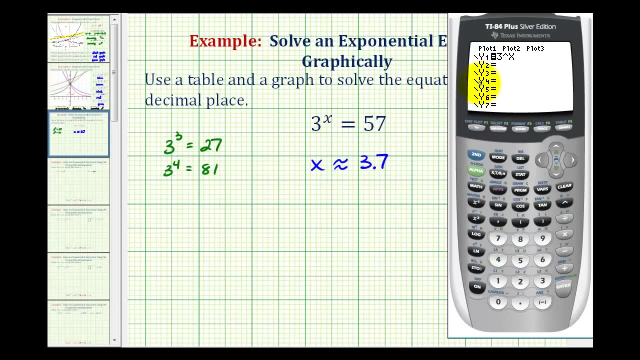 which is the closest y value to 57, at least to one decimal place. So our solution will be approximately 3.7.. And now we're also going to solve this graphically. So let's go back to the calculator, press y equals and then for y2,: 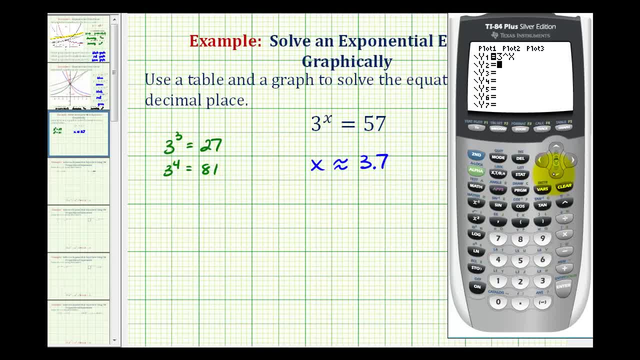 we'll enter 57, the right side of the equation. So now, what we're going to do is graph both of these equations on the same coordinate plane, and then look for the plus sign. This is the point of intersection. Before we do this, though, we have to set up the window. 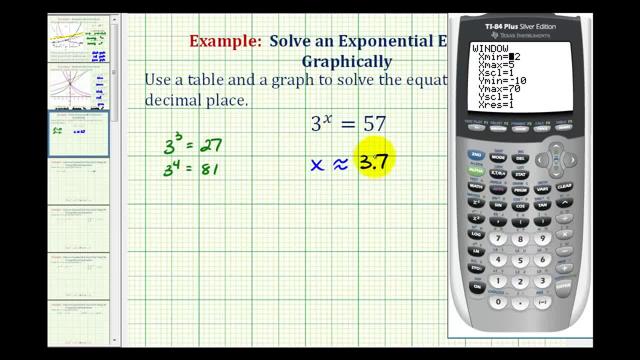 So let's press the window key. We know that we must include at least x equals 3.7 along the x axis. So notice how I have the x axis going from negative 2 to 5.. And then for the y values, we know it must include at least 57.. 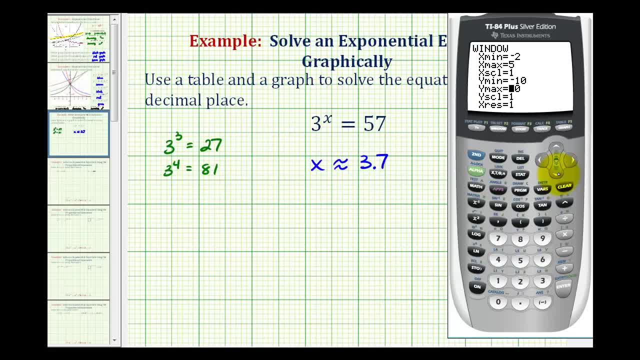 So let's go from negative 10 to 70.. Now let's go ahead and press graph. So there's our exponential function and there's our horizontal line. y equals 57.. We want to find the x-coordinate of this point of intersection. 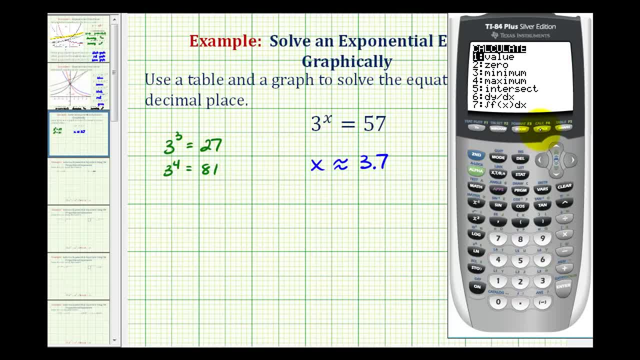 So we're going to press second trace for a calculation. We want to select option five for intersection, So we're going to just press 5.. And now we're going to press Enter three times one, two, three. so we round the x-coordinate. 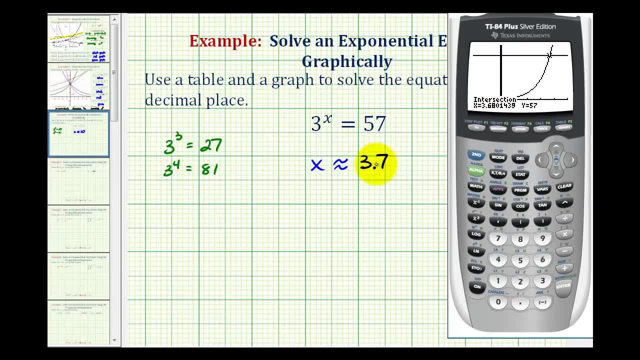 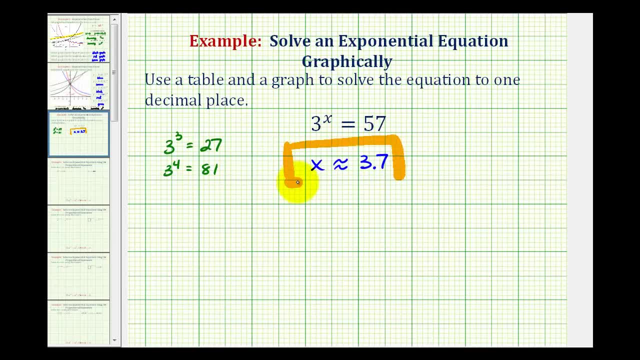 of this point of intersection to 1.5.. Okay, So at the decimal point we have the same solution where x is approximately 3.7.. Okay, I hope you found this helpful.